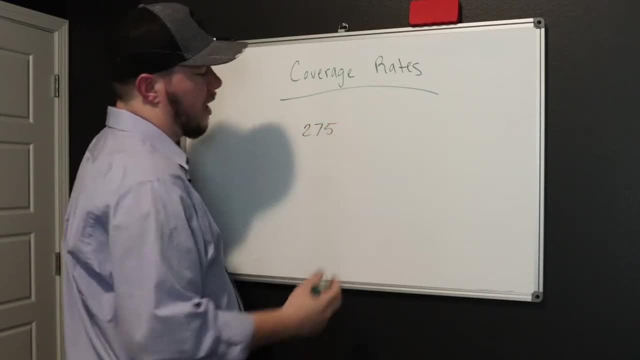 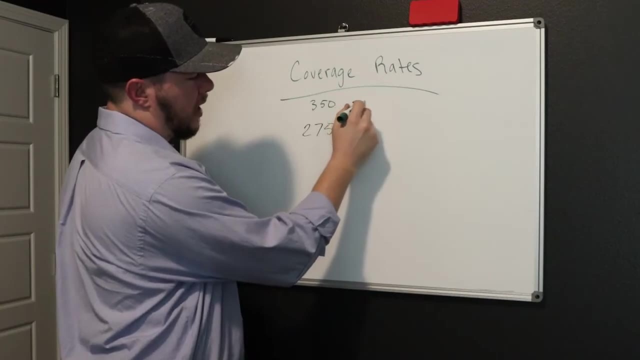 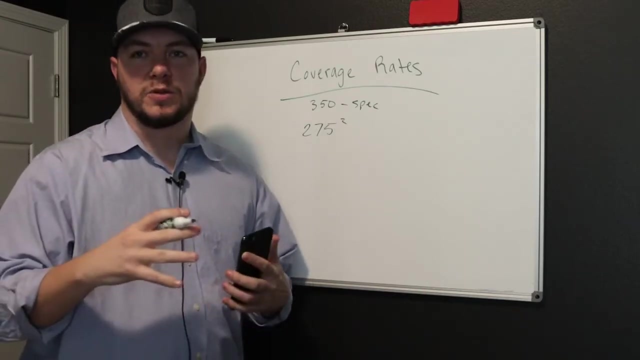 275.. So that's what we're going to work with. If the spec sheet says 350, I'm usually going to go down to about 275 square feet a gallon. You always want to have an excess of square footage or an excess of material rather over what they say. I don't really trust what the spec sheets say. 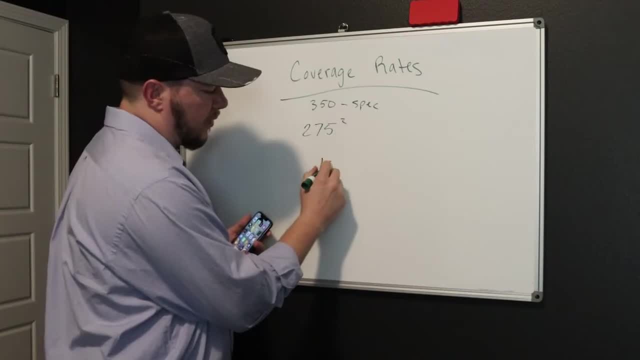 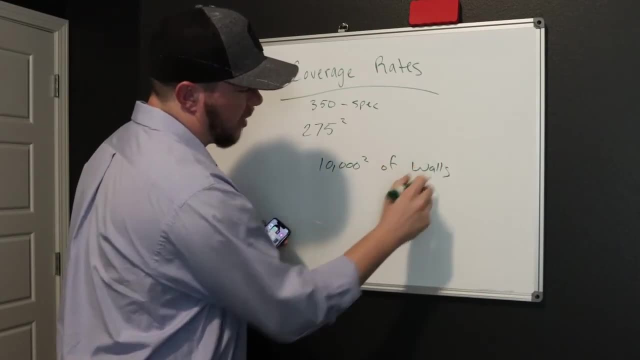 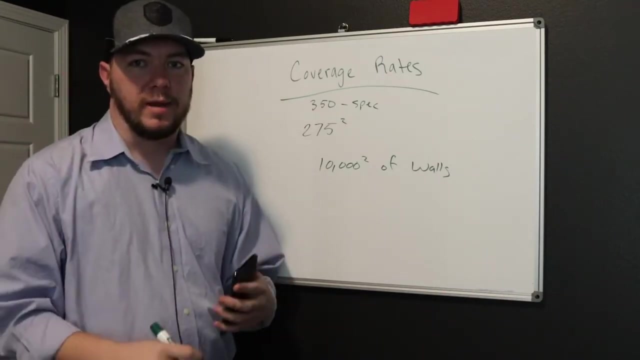 So let's do a little math. Let's say we have 10,000 square feet of walls, 10,000 square feet of walls that need to be painted. We're getting a coverage rate of 275 a gallon. That leaves us a little bit extra, you know, a little bit in the bottom of the can. 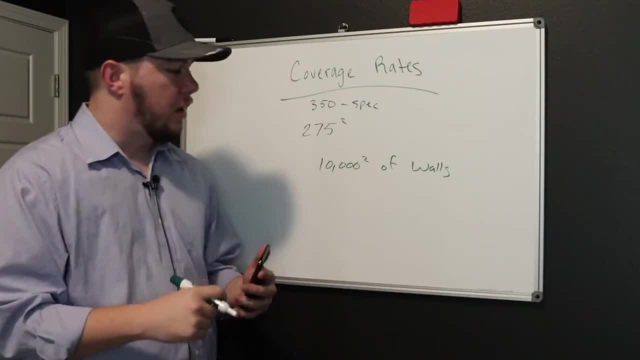 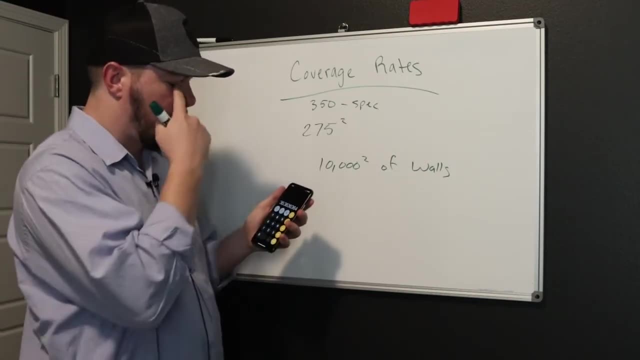 a little bit in the roller pan, a little bit in the five gallon bucket, So just to be safe. So 10,000 square feet of wall space, you divide that by 275.. That's going to be 36.36 gallons. 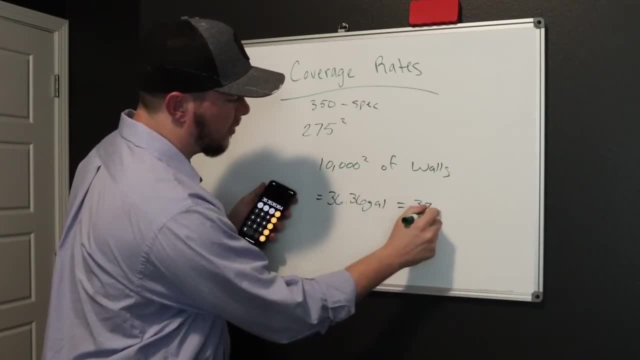 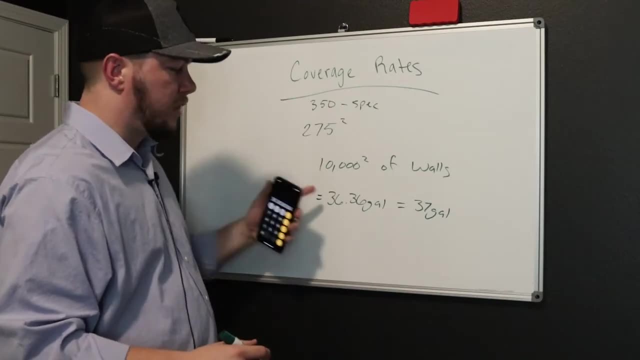 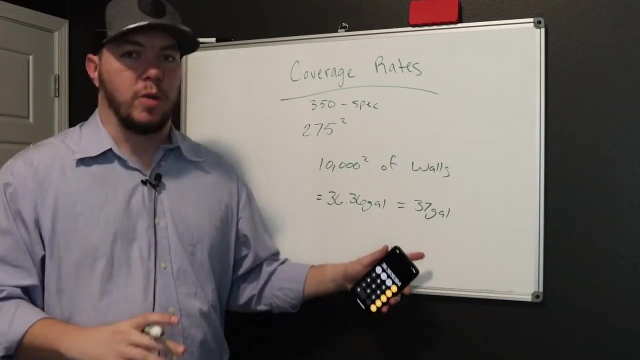 So I round up 37 gallons. So 37 gallons of product at a 275 square foot, a gallon coverage rate is going to mean you're going to need 37 gallons. But before you stop there you need to realize that that's only one coat, So that's one coat. If you're going to do two coats, you need to double. 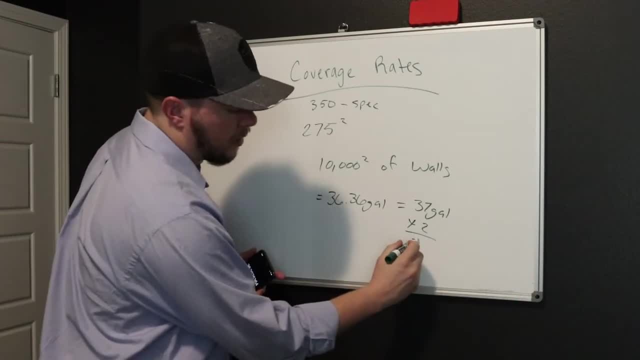 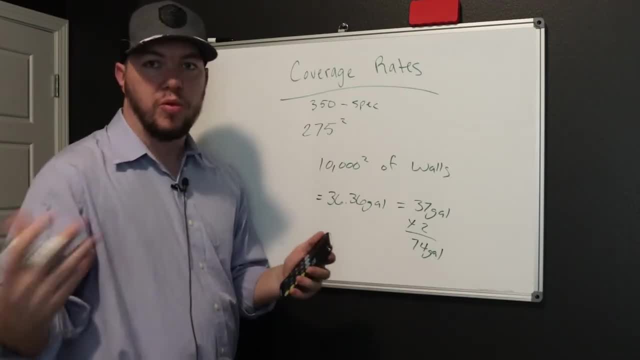 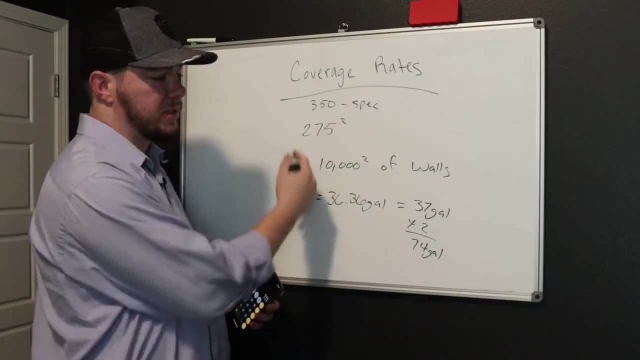 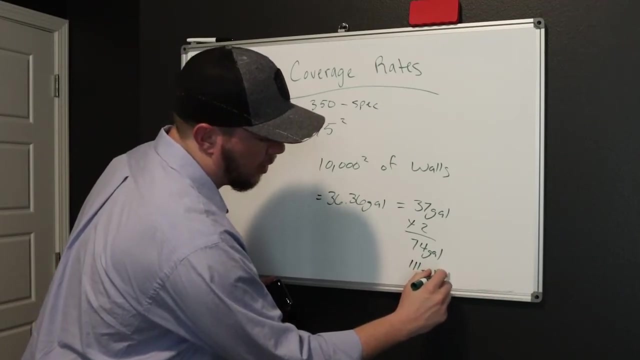 So that's three If it's going to take primer as well. So if it's going to take primer and the primer has, you know, the same coverage rate, let's just assume for the simple map the primer has the same coverage rate, you're going to need 111 gallons at three coats. at two coats. So 37 gallons is that one coat? 74 gallons at two coats, 111 gallons at three coats, And this will give you exactly what you'll need for, let's say, everything is going the same color. You can use this formula here. 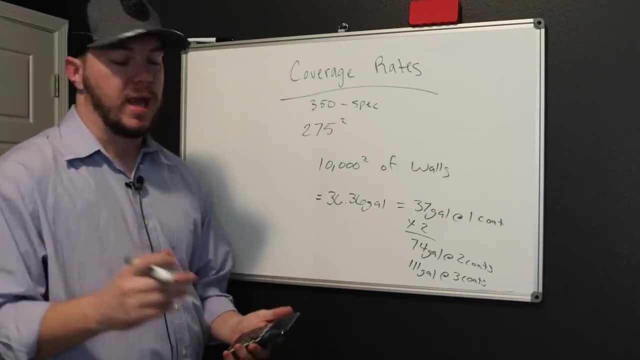 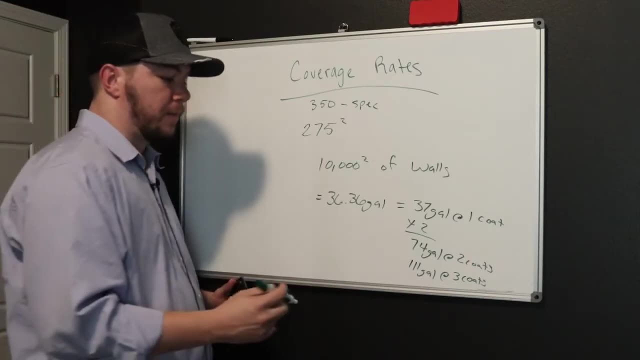 this little simple math equation and you can tell exactly how many gallons of paint you'll need for a given situation, for walls or ceilings or anything flat like floors as well- Talking concrete sealer, As long as you know what your coverage rate is. you just come down a little bit off of it. This is the coverage rate I would go by. if it said 350, I'd go 275 a gallon. If it says 500, I'd go 400 a gallon. You kind of just ballpark.